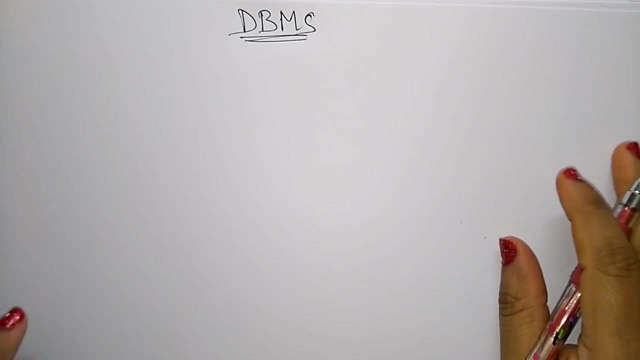 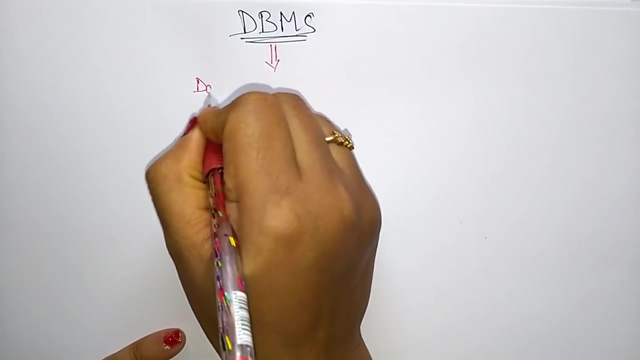 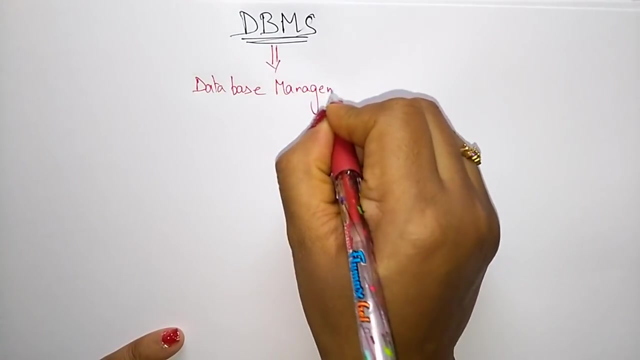 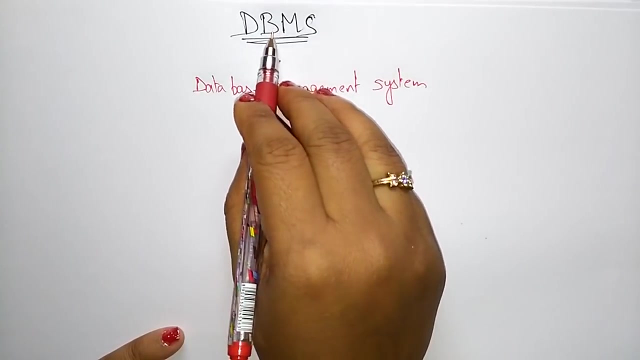 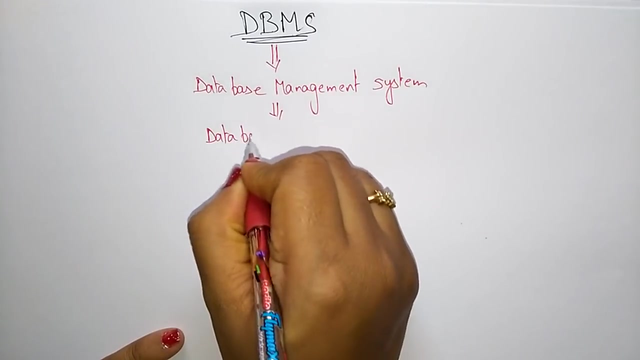 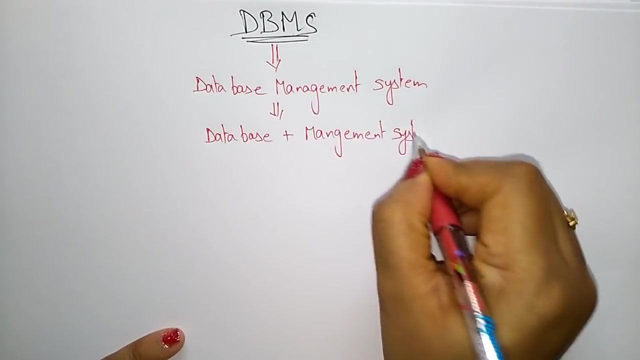 Hi students. coming to the next subject, database management system. So let us see the introduction part of the database management system. So actually this database management system stands DBMS stands as database management system. So DBMS D means database management system. So we can break this like database plus management system. So this is a two word: database and management system. 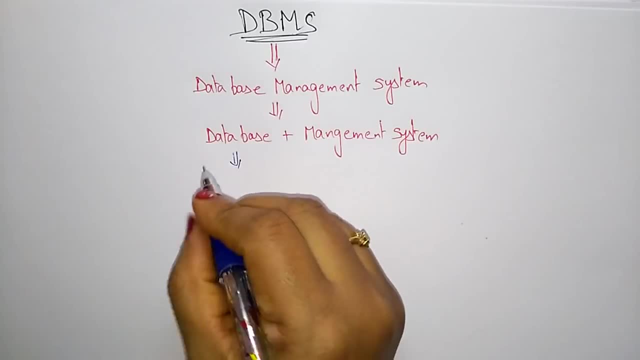 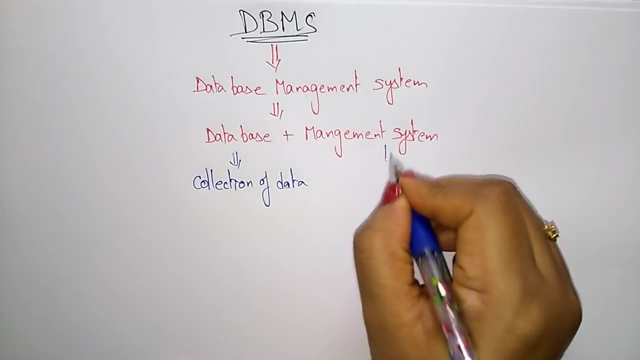 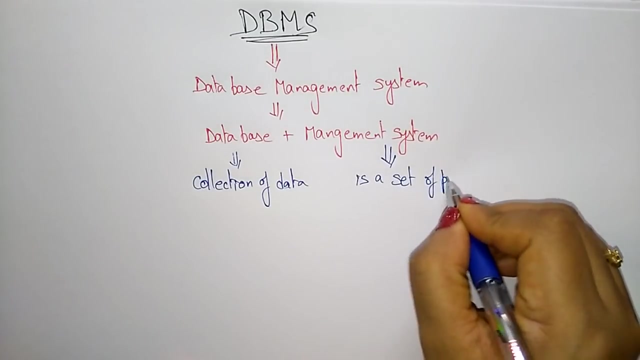 So a database is nothing, but it is a collection of data. So database is a collection of data. Then what about the management system? Management system is a set of programs. Management system is a set of program to store and retrieve those data, Those data that is present in the database. 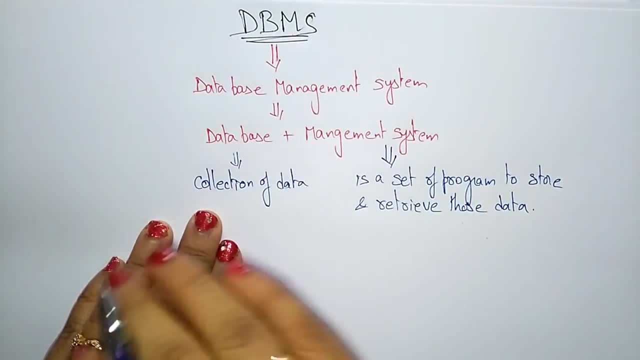 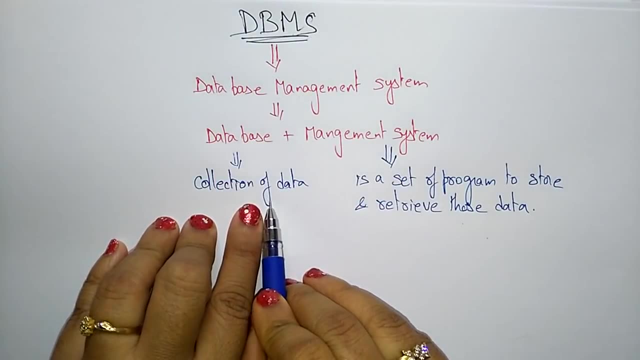 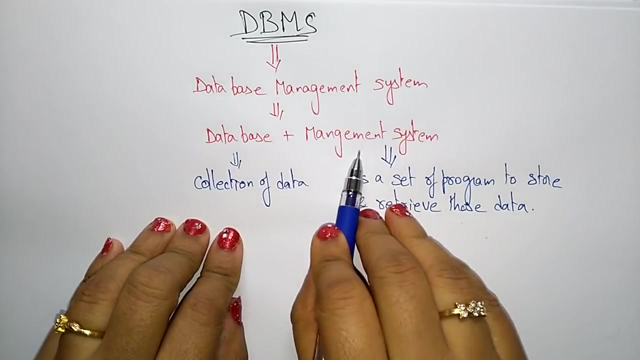 So this is a combination of the database management system. So it's a simple word: a database management system. So database management system is nothing but it is a collection of data which performs set of operations like retrieving data, storing data, like that. So management system is a set of programs that store and retrieve those data. 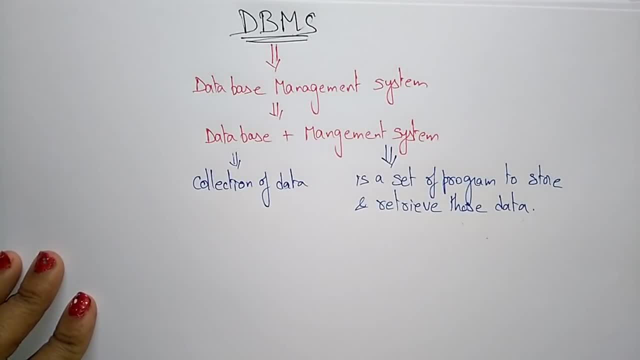 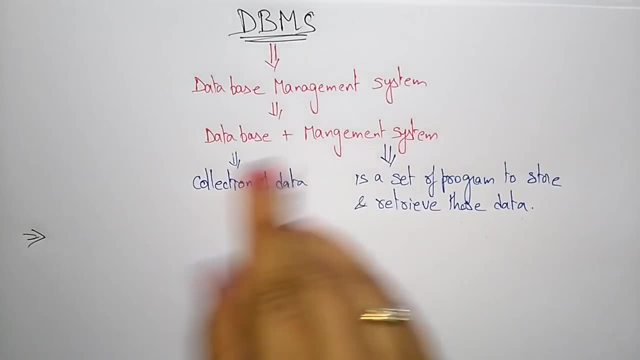 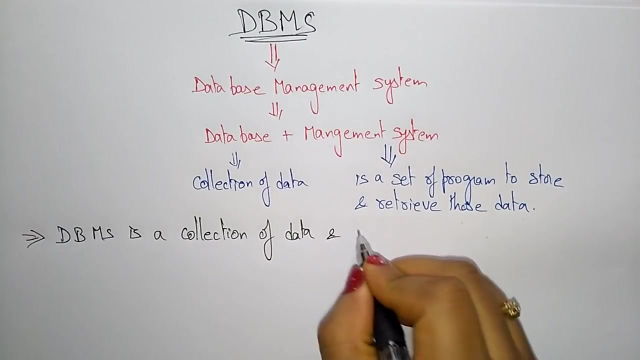 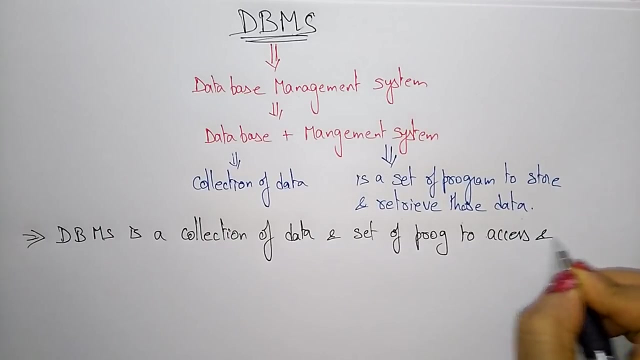 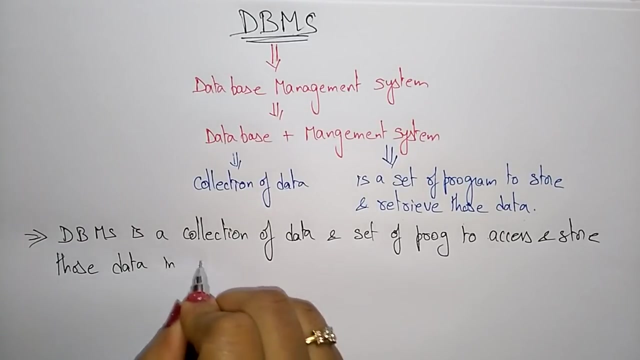 So based on this we can define. So now I'm writing the definition of database management system. So based on this I can say DBMS is a database management system: Collection of data and set of programs to access and store those data in an easy and efficient manner. 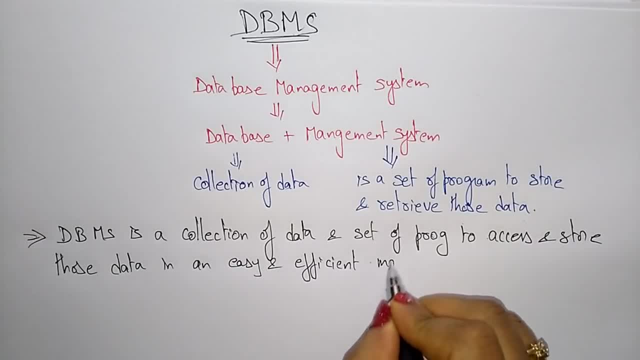 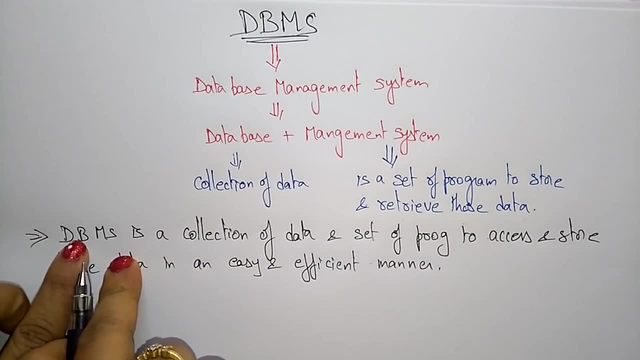 So this is the definition of the formal definition of database management system. So it is a collection of data, So the name itself is indicating. So database it is a collection of data, and management system is a set of programs to access and store those data in an easy and efficient manner. 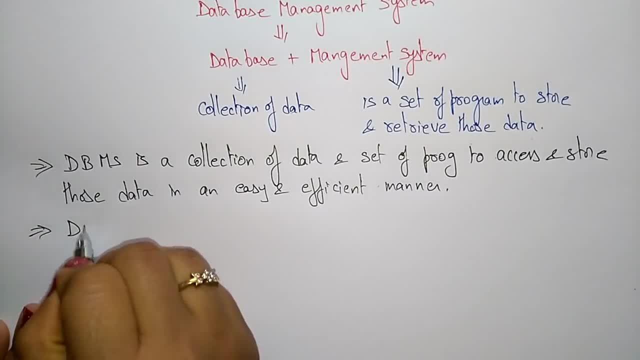 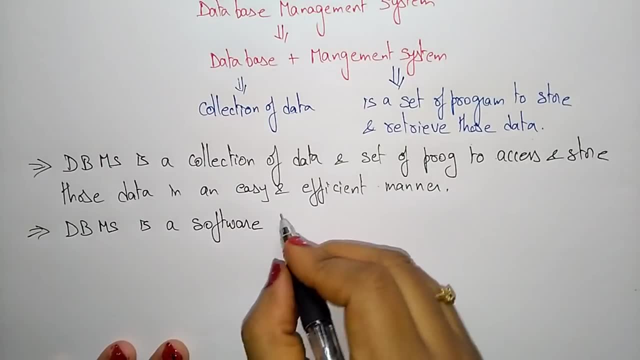 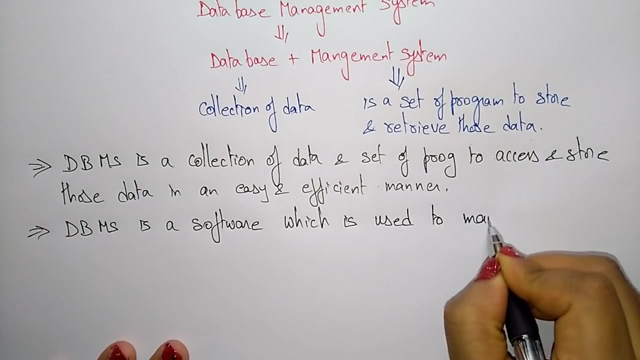 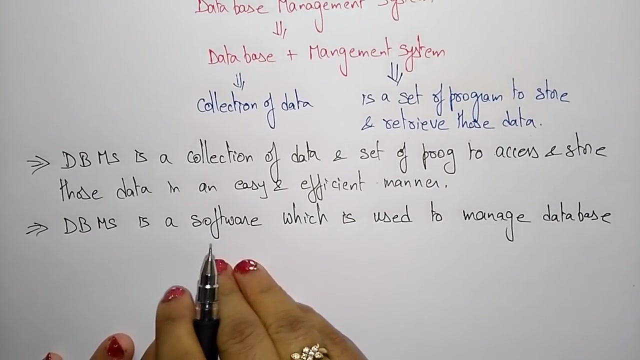 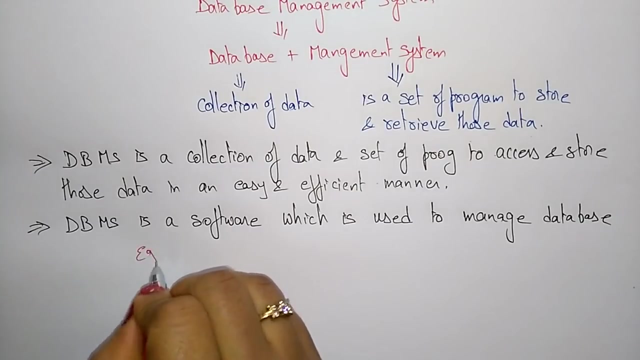 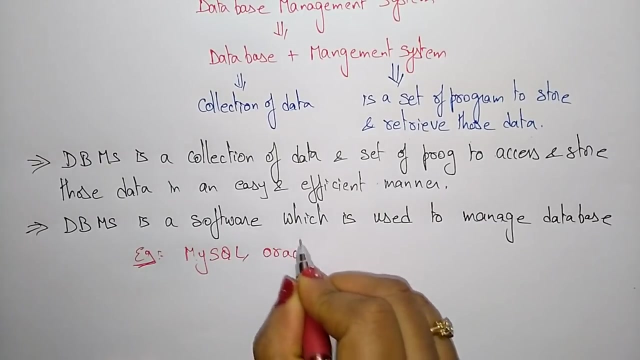 So you can also say: database management system is a software, Is a software Which is used, Which is used to manage the database. So to manage database we need a software, That software you call it as a database management system. So examples for this database management system, the softwares are MySQL, Oracle, etc. 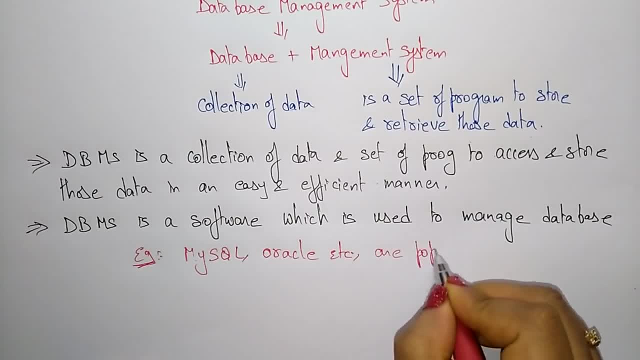 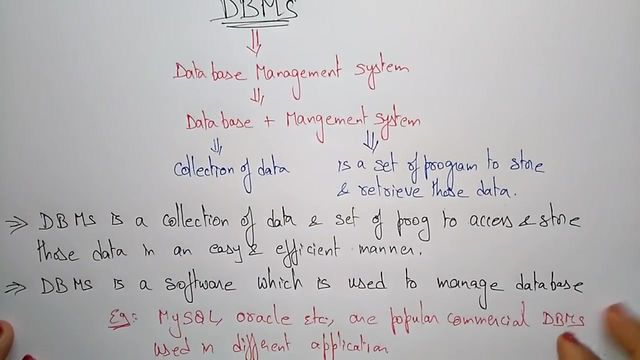 So these are the popular commercial database management system software used in different applications. So this is a formal definitions of the database management system. So DBMS is nothing but it is a collection of data and a set of programs to access and store those data. 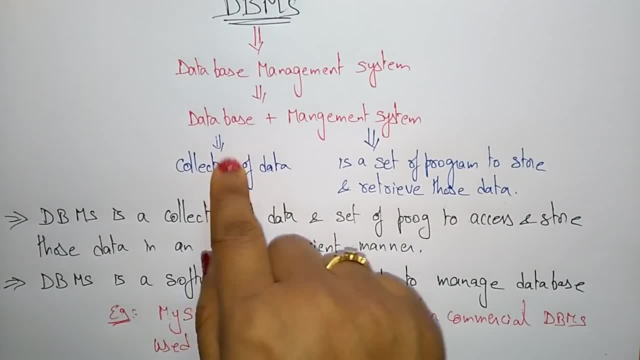 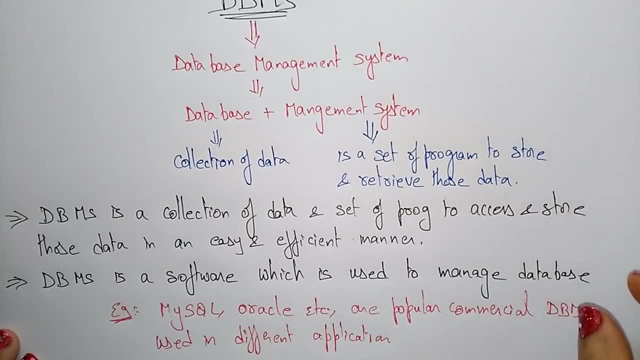 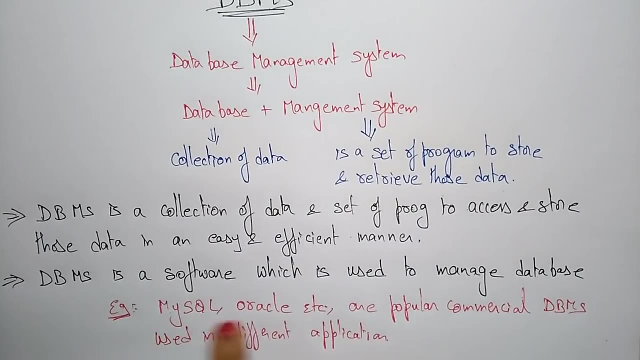 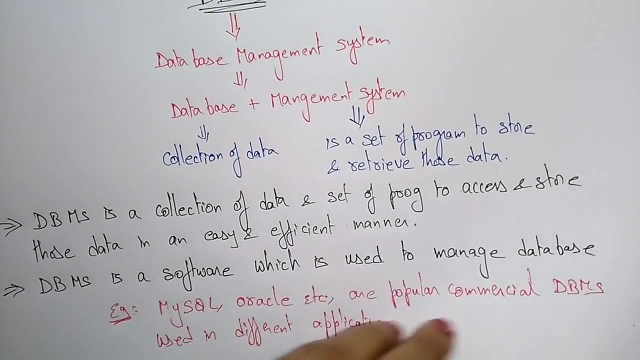 So it uses programs to access and store the retrieve the data in an easy and efficient manner. we call it as a database management system. So this is theと思います being discussed earlier and then As, and it can also say it is a software. 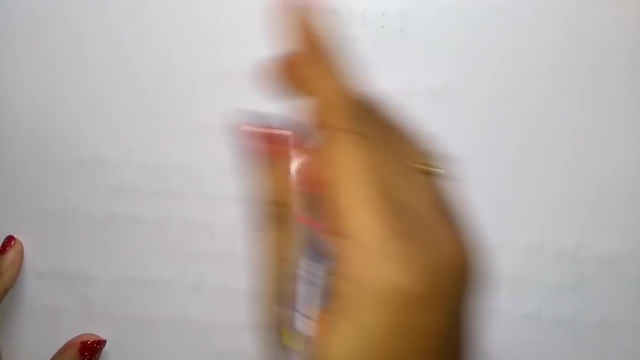 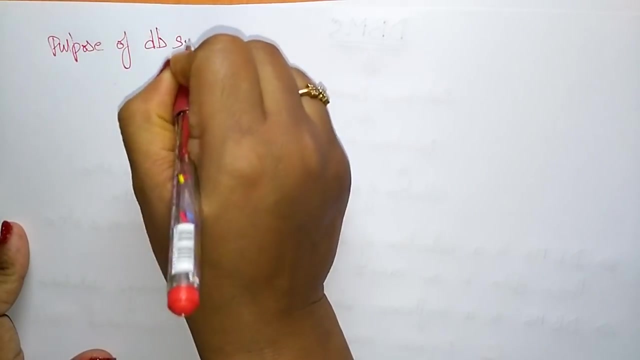 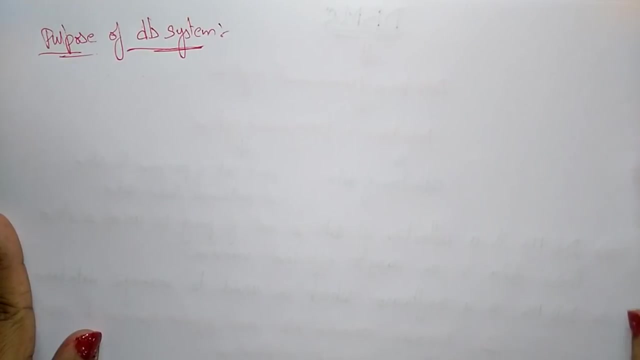 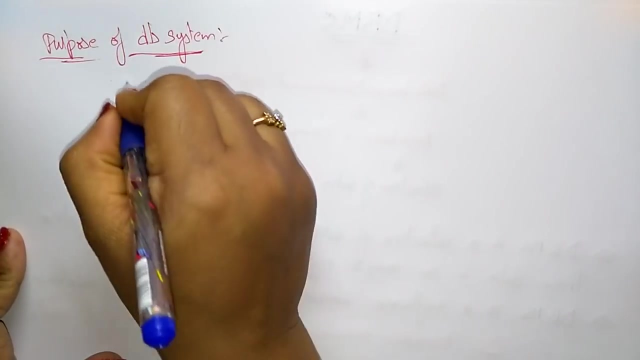 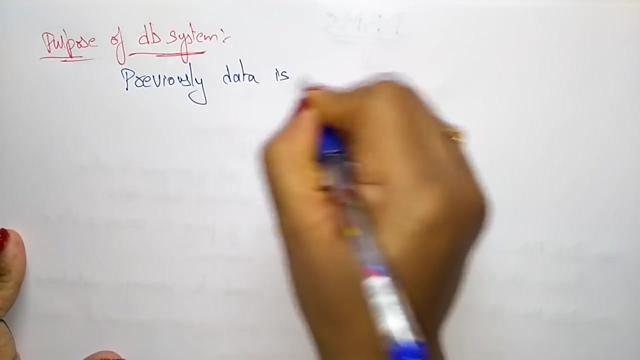 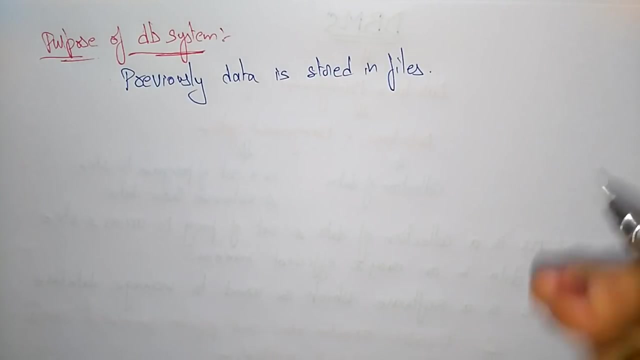 what is the need of using the database system? purpose of database system. so why we are going for database system for storing the data. so actually in earlier days, a database application store in an file system. so previously, previously, data is stored in files. so already we know that the data is stored in files. 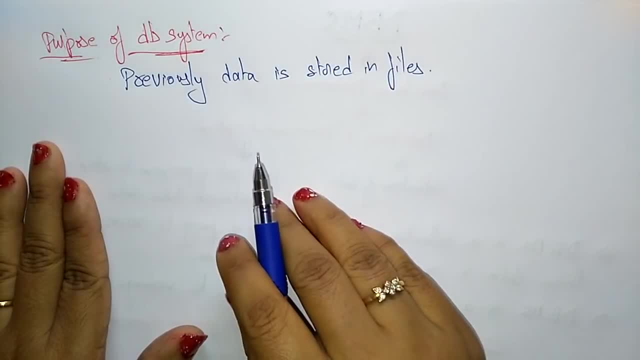 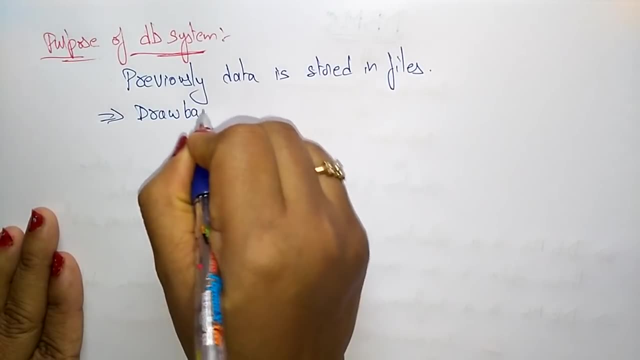 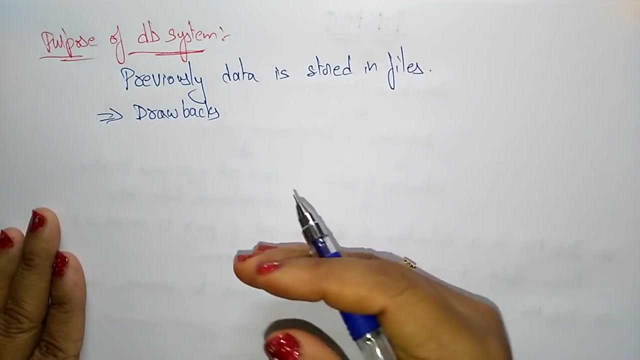 but instead of using the files, why we are going for the database system? because these file system is having some drawbacks. so if you know the drawbacks of the file system, then you will need the purpose of the. then you will know the purpose of the file system. then you will know the purpose of the file system. 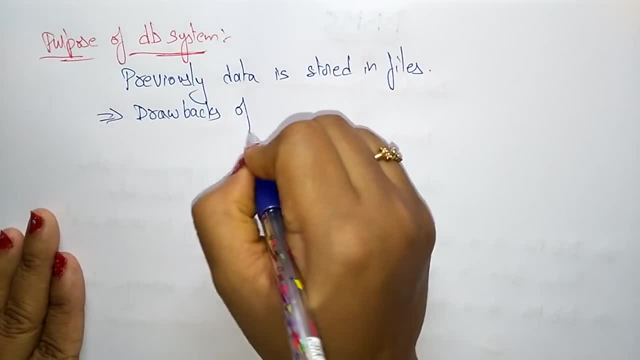 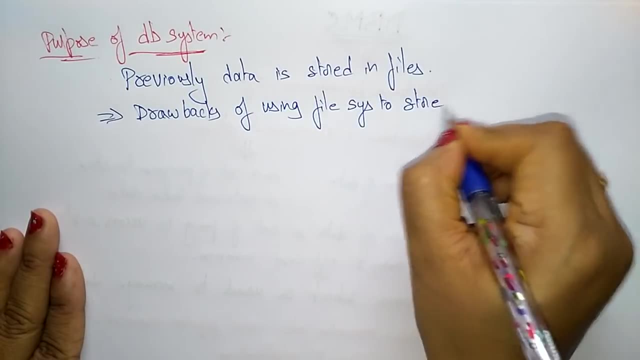 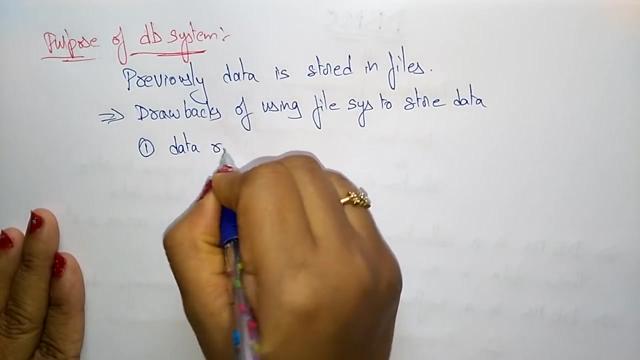 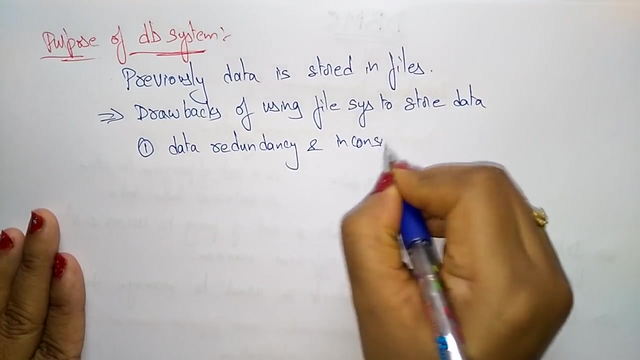 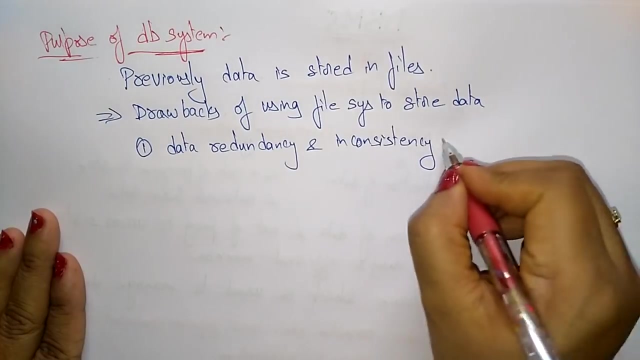 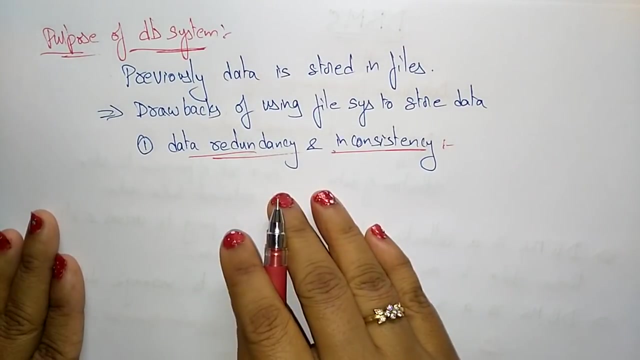 purpose of the database system. so the drawbacks of using file system to store data, or first one, the rate data redundancy problem and inconsistency. so this is the first drawback in file system. so data redundancy and inconsistency means data redundancy means here the duplication of information in different files. so in different file, some different. 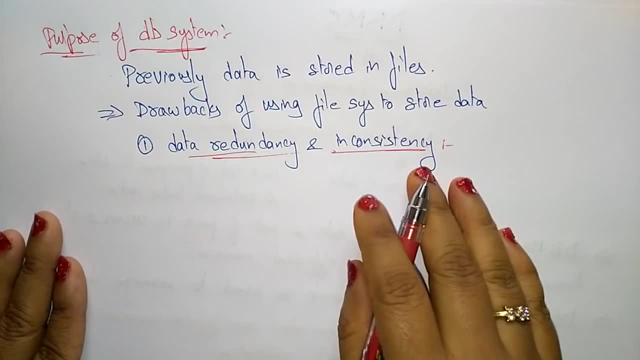 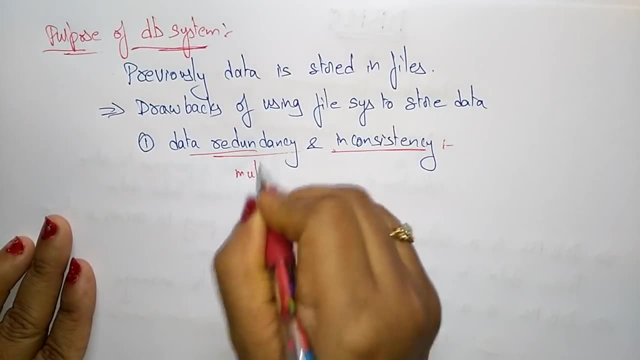 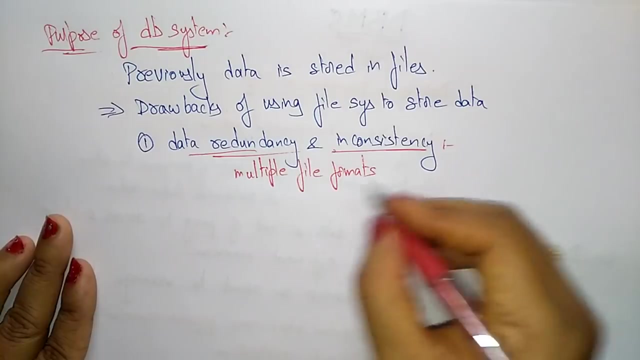 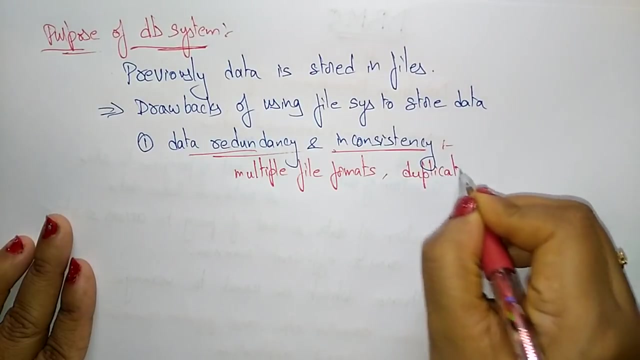 duplications will be there and also multiple files formats will be there, so that will that is, a data redundancy and inconsistency. let me write: multiple file formats will be there so that the data will becomes a inconsistency. file formats and duplication of information in different files so that 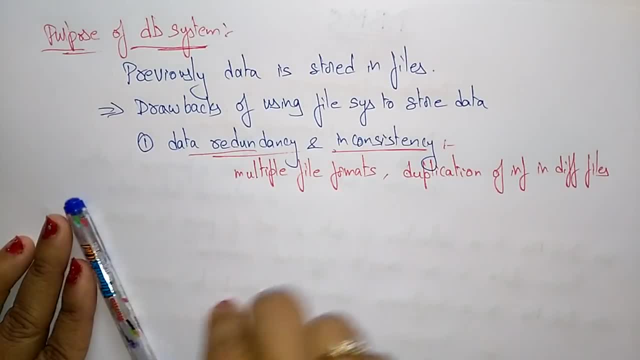 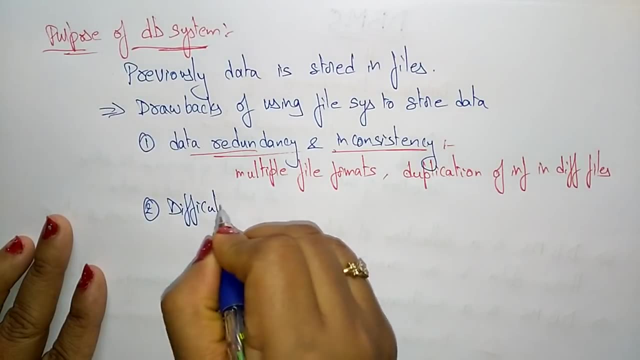 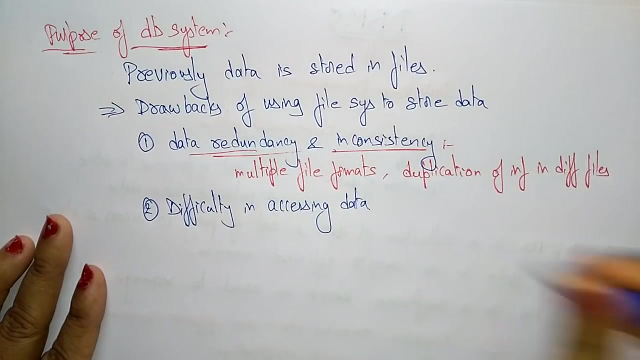 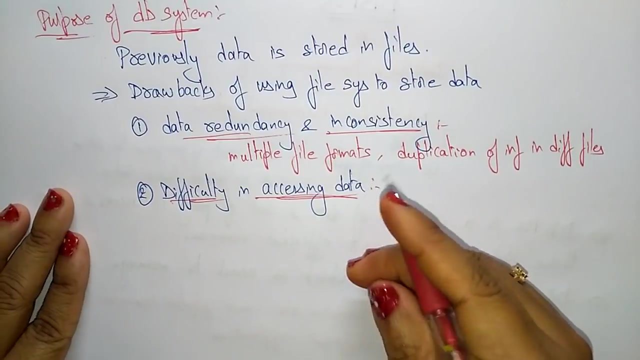 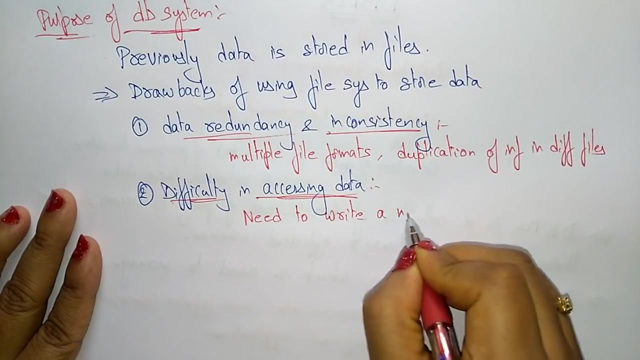 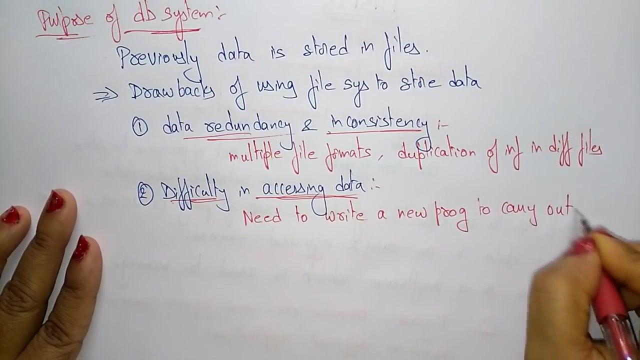 is one of the drawback in file system. and next difficulty: difficulty in accessing data. so to access data in file system is somewhat difficult. why it is difficult? why it is difficult to access the data in file system? because sometimes it need to write a new program, new programs to carry out, carry out each. 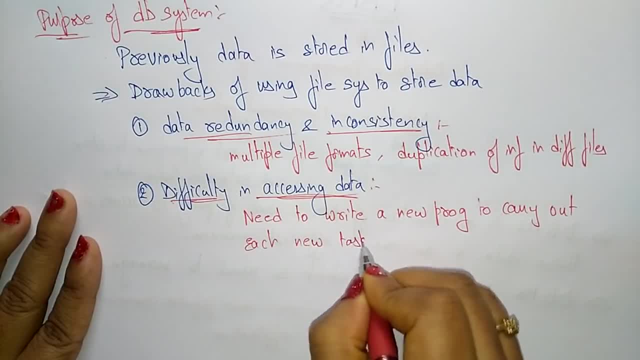 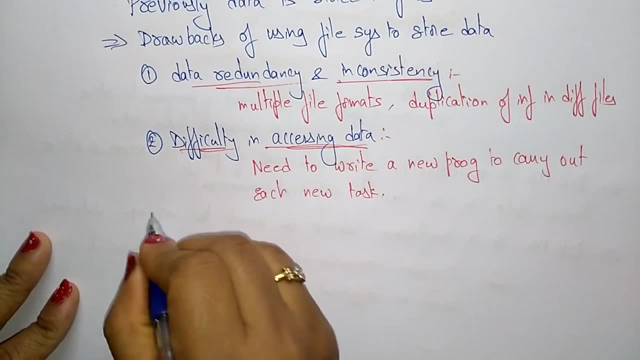 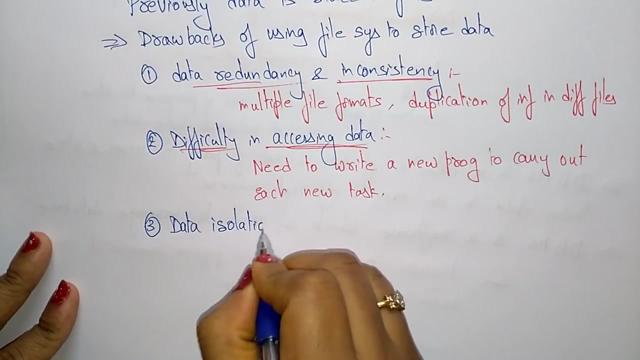 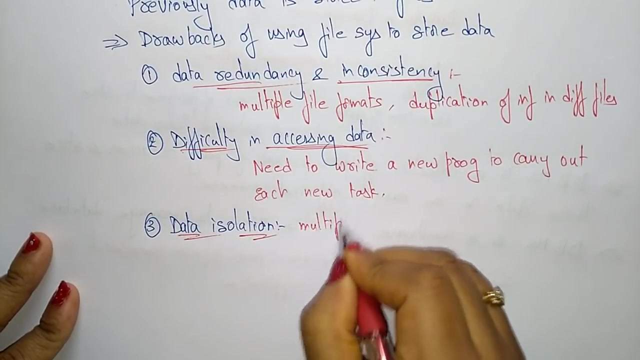 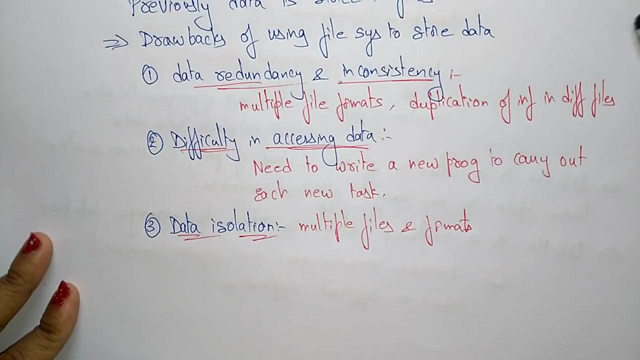 new task. so in that cases the file system is difficult to access the data. next, data isolation. then another problem in using the file system is data isolation. so here the data isolation means it will use a multiple files, multiple files and formats. next it's having the data security problem. data security, so when? 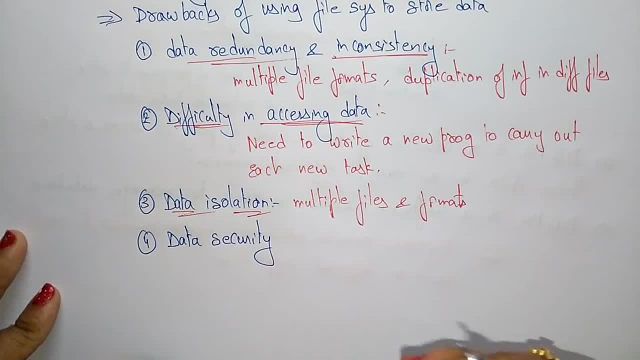 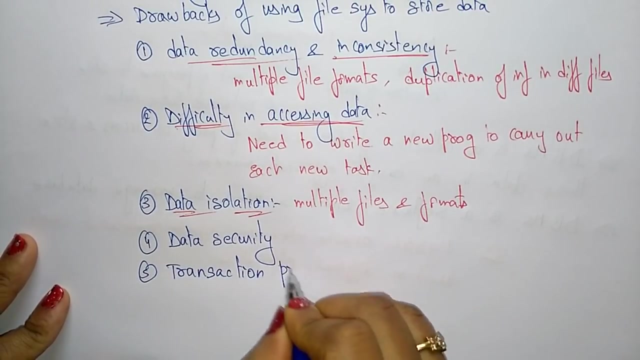 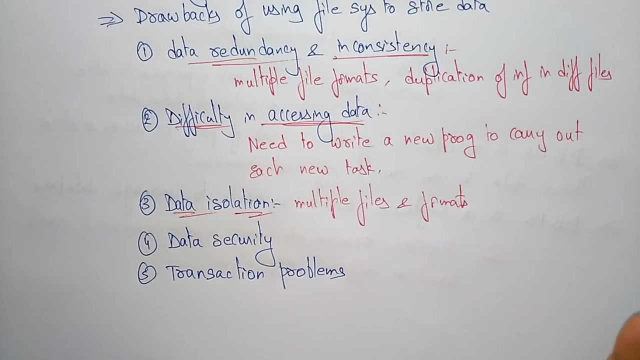 And if you store the data in files- retrieving and storing the data is somewhat some security problem issues will be arised in file system And transaction problems will be there. Transaction problems If you want to transfer the data from one source to another. another means source to destination.